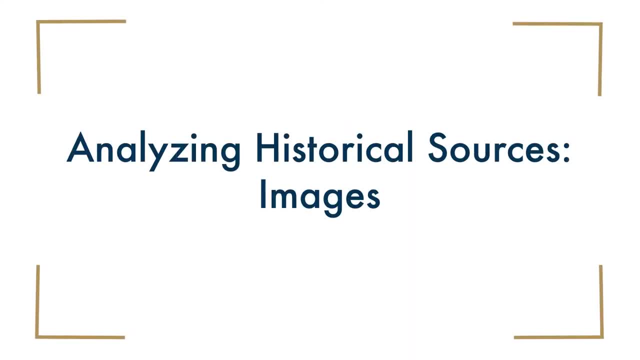 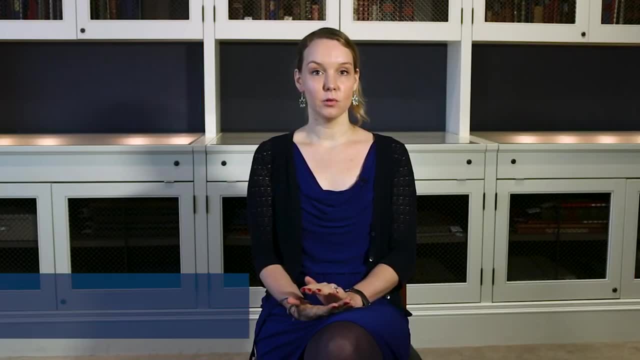 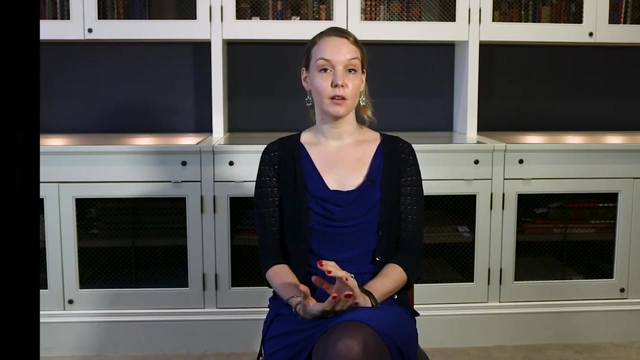 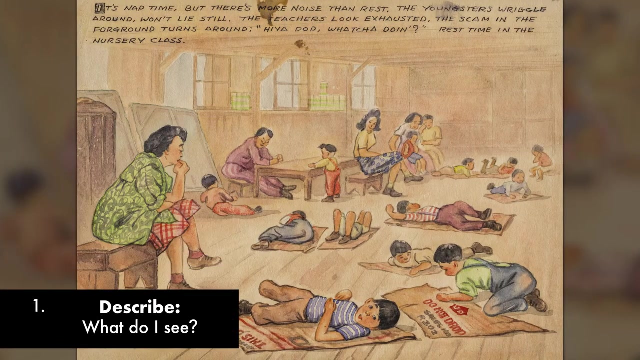 When you're presented with a visual source and you know that this visual source is a historical document or part of a historical document, there are roughly three steps that you might take in reading it. So, for example, let's look at this image First, describe. 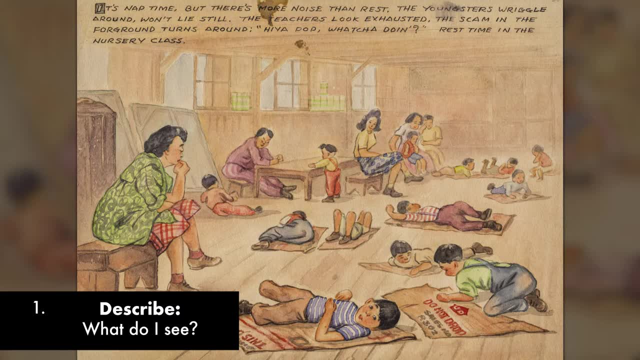 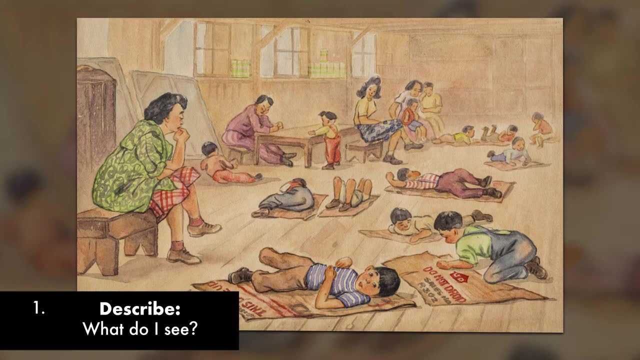 what you are seeing. Look at the image itself. Do not be distracted by the caption. Just vocalize or write in a brief paragraph the things that you notice: the colors, the angles, the perspective, what you think it might depict. That's what you want to do first, before. 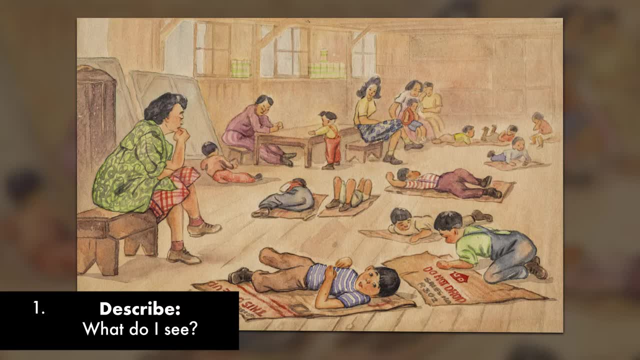 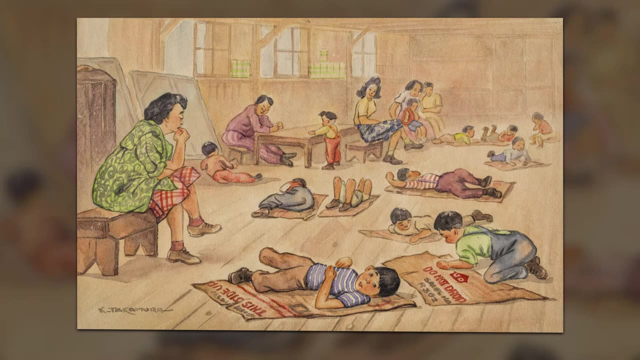 looking at any caption or text that might influence your perspective, It's easy to miss things if you allow the written text to determine what you see. One thing you might notice about this watercolor, without any additional information, is that no one is posing. It's not a portrait. It's not a political pamphlet. This is a moment. 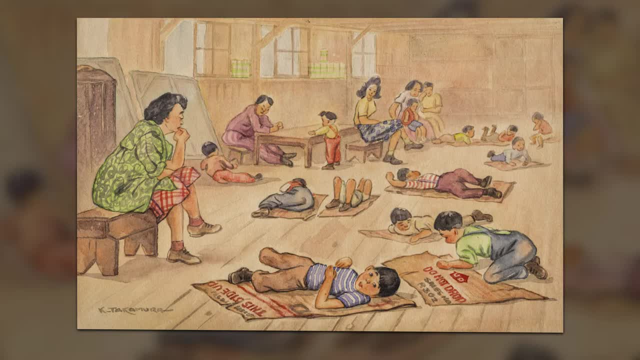 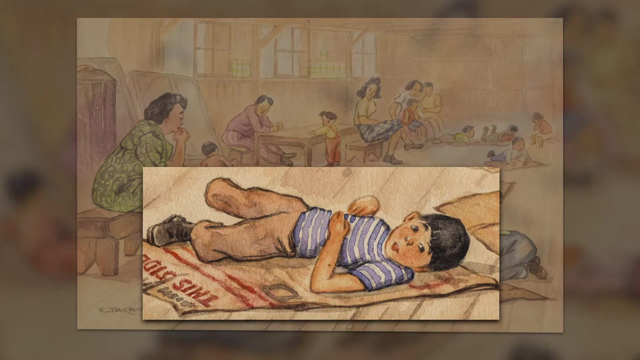 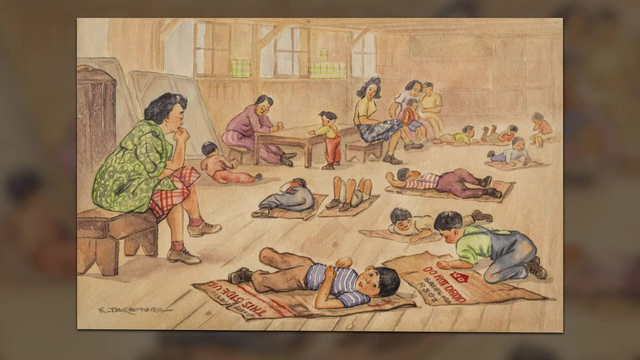 from everyday life. No one seems disturbed by the artist's presence. In fact, the only hint we get that the artist was part of the action here is that in the foreground we see a boy on the floor looking directly at the picture. The scene itself appears to be of a group of women watching young children, some of 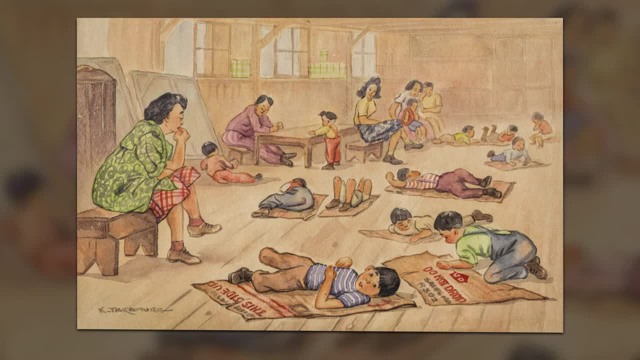 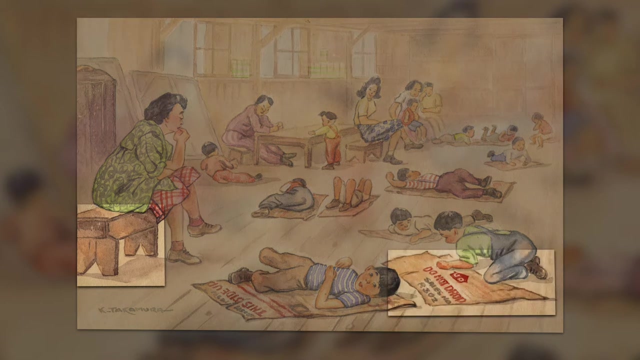 whom are asleep, some of whom are playing. They all appear to be of Asian descent. We can also see that they're all in a very sparsely decorated room: Wooden floors, wooden benches, cardboard boxes, no toys or anything you might expect to see for children. this 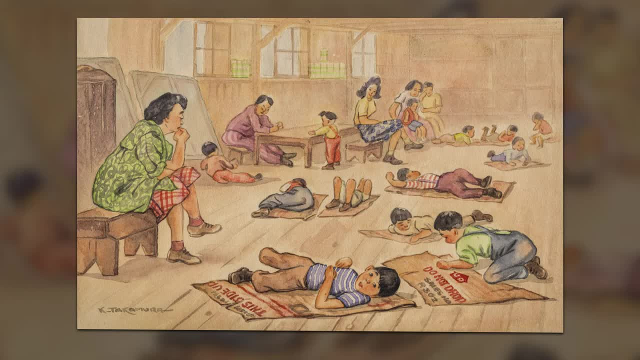 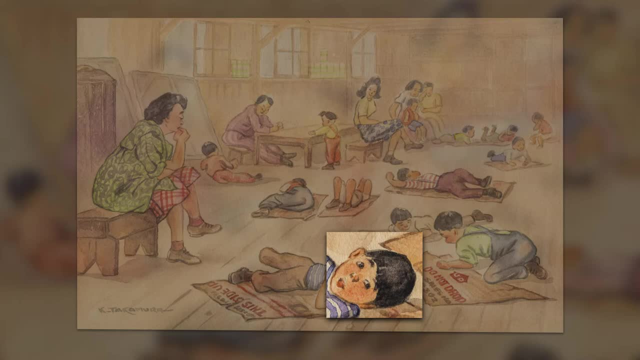 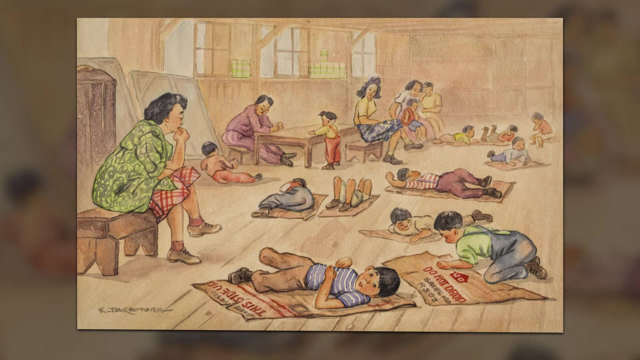 age. There are also no real, discernible facial expressions. The boy in the foreground looks intrigued, playfully sticking out his tongue, but beyond him there's no distinct mood or tone to the watercolor, Nothing particularly happy or sad, confrontational. 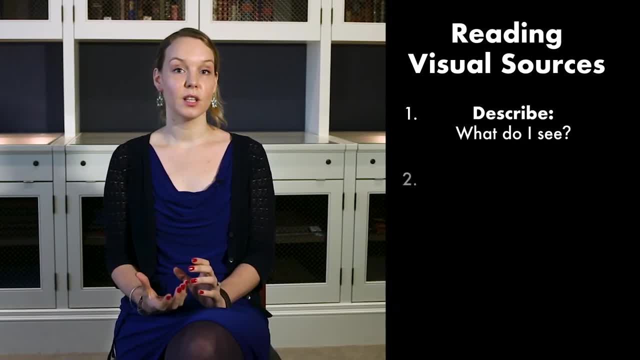 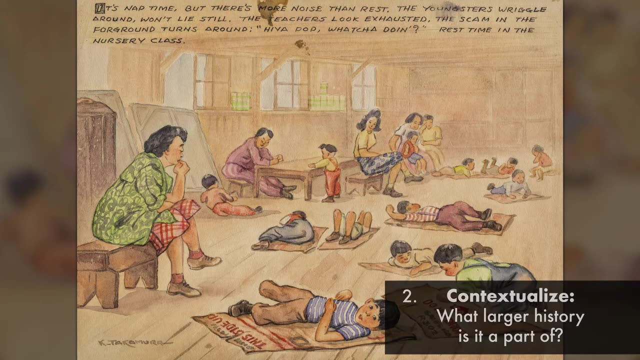 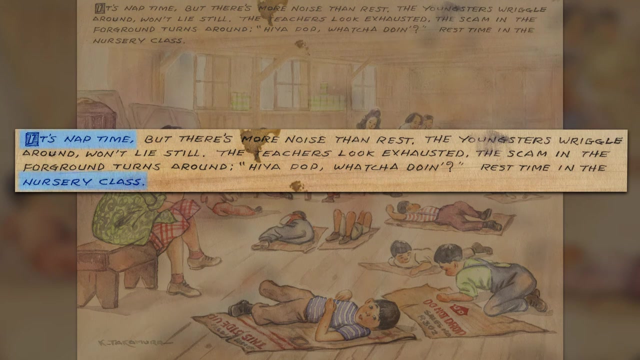 Second, once you've done this quick surface-level reading of the image, you can start looking at what it might depict. So here we get lucky, because this watercolor actually has quite a lot of info for us. We learn from the caption that it is indeed a very ordinary scene: nap time at a nursery. 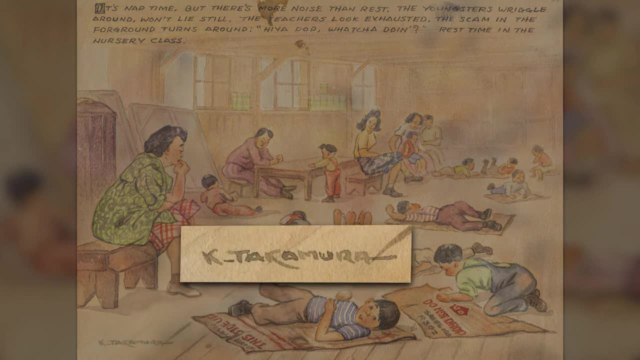 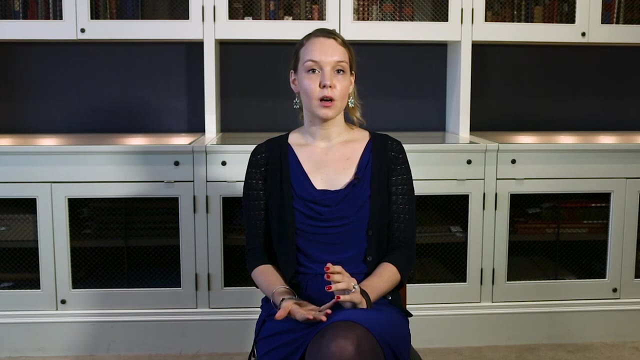 But what's also of interest is that we get the name of the artist, Kengo Takamura, and we also get a title for this watercolor. The title is not on the front of the watercolor, but you would be able to see it if you found. 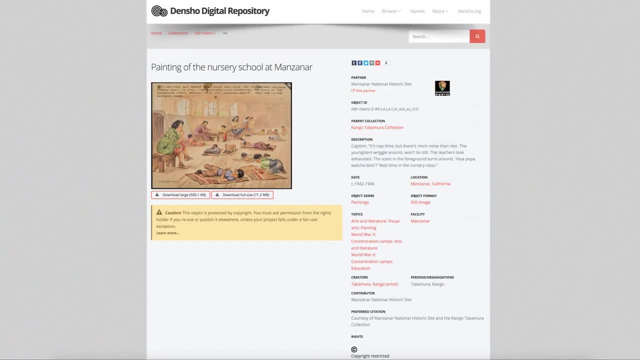 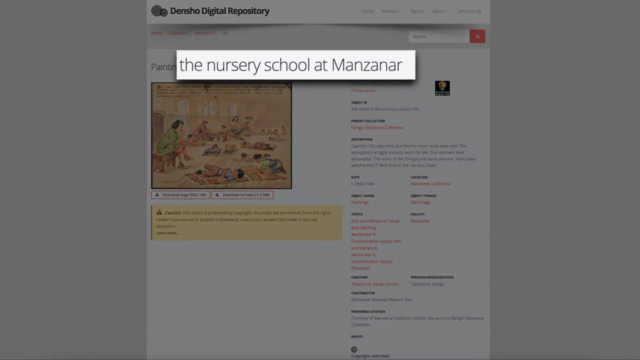 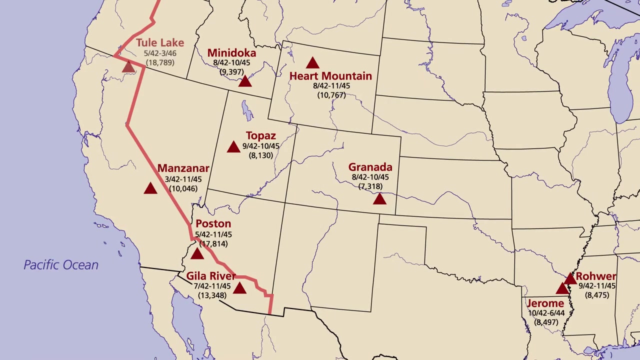 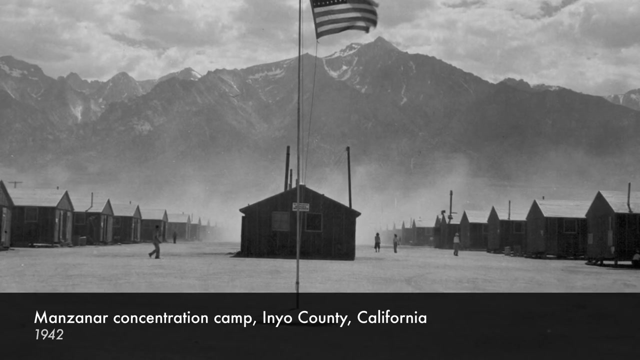 the image on Lightroomcom, The watercolor is called The Nursery School at Manzanar. Now you can start fitting in historical context. We know that Manzanar was one of ten concentration camps where Japanese Americans living on the West Coast were incarcerated during World War II. Most of them were citizens. Note that. 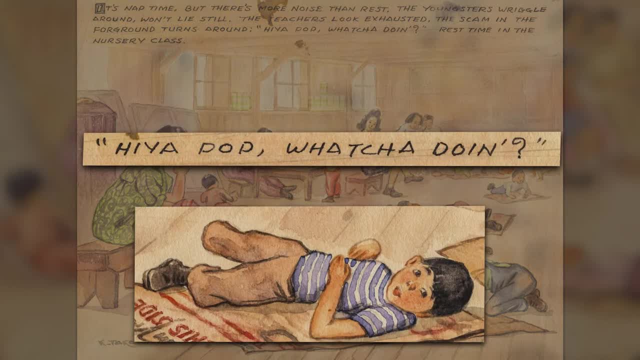 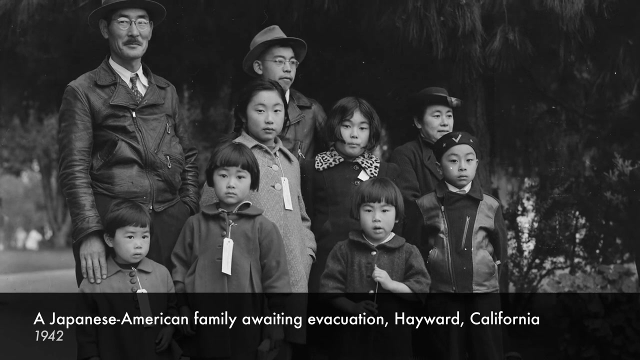 the boy asks Hiya pops whatcha doing? In distinctly colloquial or everyday English. So we can assume he was born and raised in the US. Nevertheless, after Pearl Harbor anyone of Japanese descent, citizens or not, were accused. 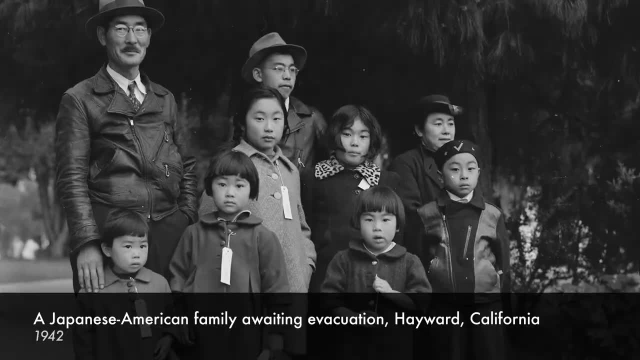 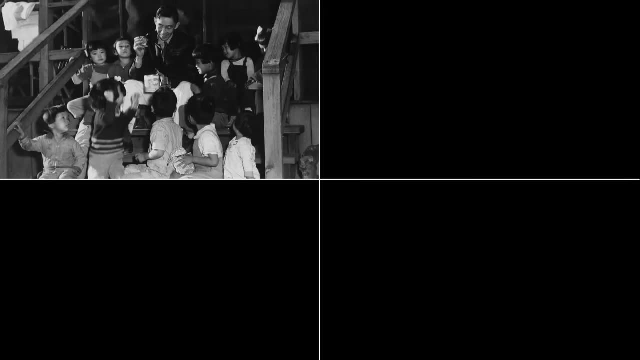 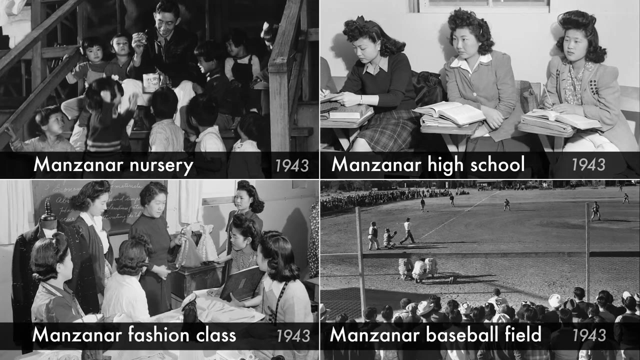 of being enemy aliens without any evidence. Manzanar, like many of the other camps, tried to preserve a sense of normalcy by running a nursery school, a high school, classes for adults, etc. But clearly this all had to take place through improvisation, as the camps were makeshift. 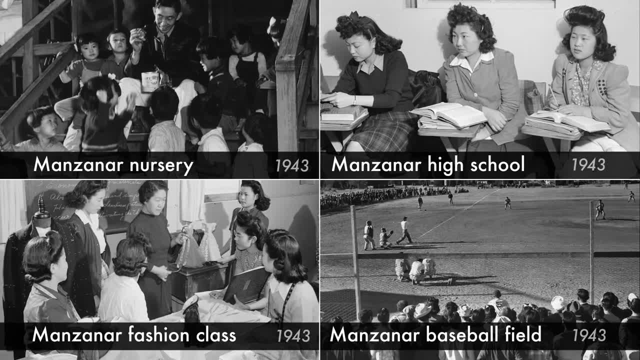 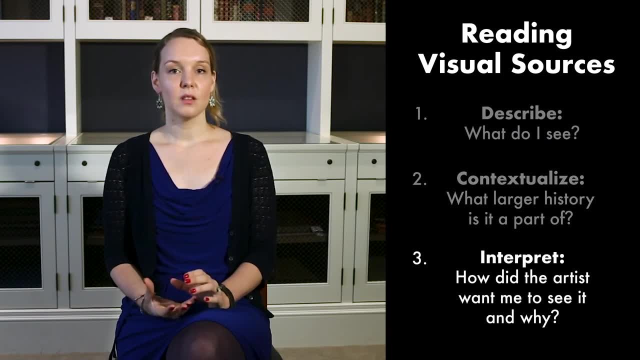 sometimes converted horse stables or hastily constructed barracks. Now for your final step. you can try to figure out why the artist made this watercolor, how he depicted the specific scene and what we can learn from both of these things combined that might tell us something about, in this case, Japanese inclusion. 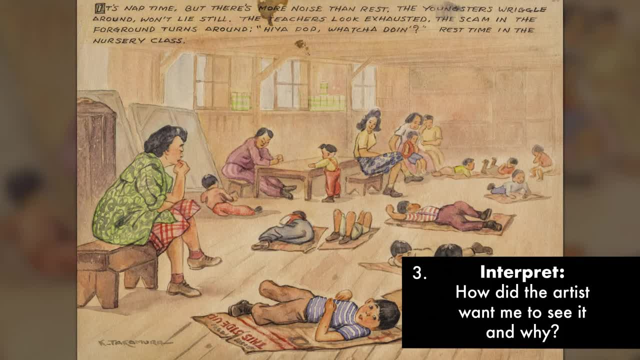 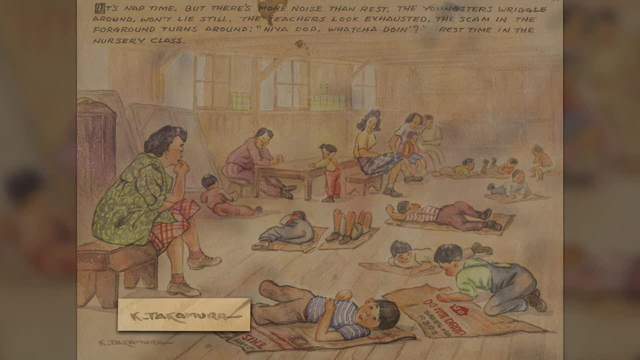 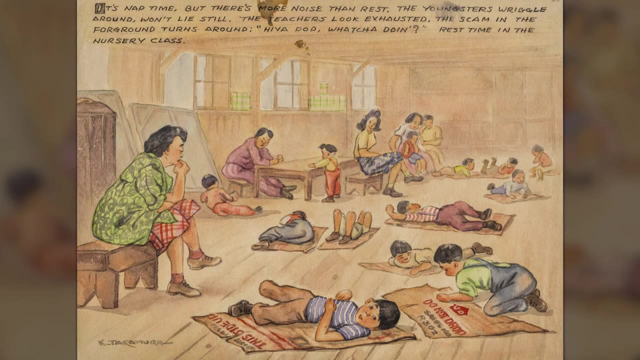 We already saw by the perspective of the watercolor that the artist was part of the scene depicted. His name, Takamura, confirms to us that he was likely also incarcerated at Manzanar. This helps explain why it is a watercolor. The people in the camps were. 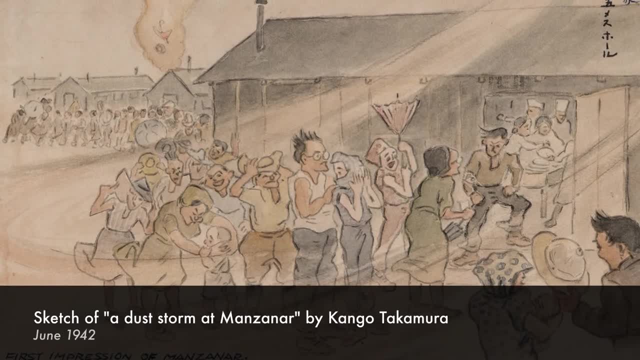 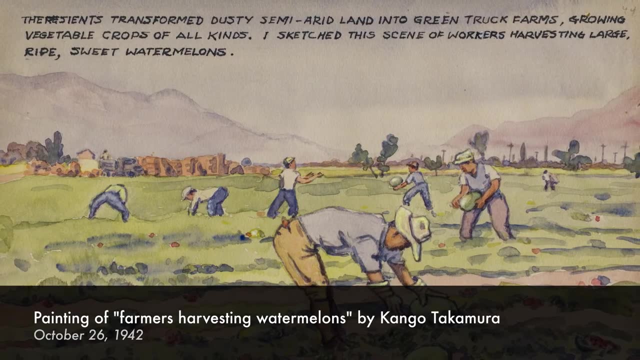 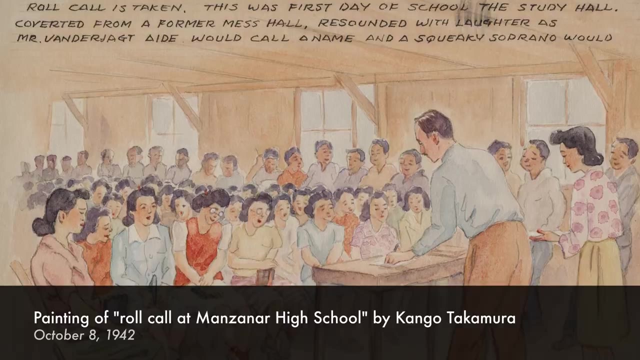 forbidden from taking any photographs or video to document their experiences, so some of them took to other artists to document their experiences. They also took to other art forms like cartoons, watercolors, paintings, sketches, to record life from within the camps. Many of them wanted to keep evidence of the injustice brought.